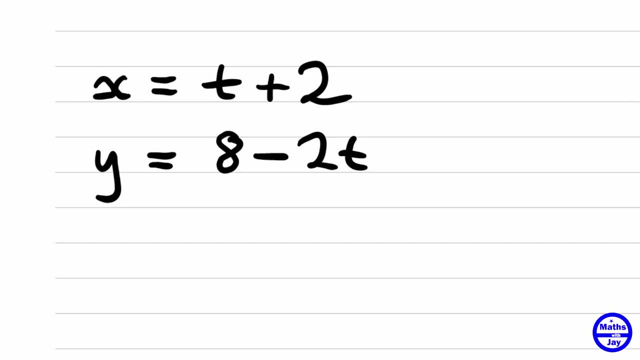 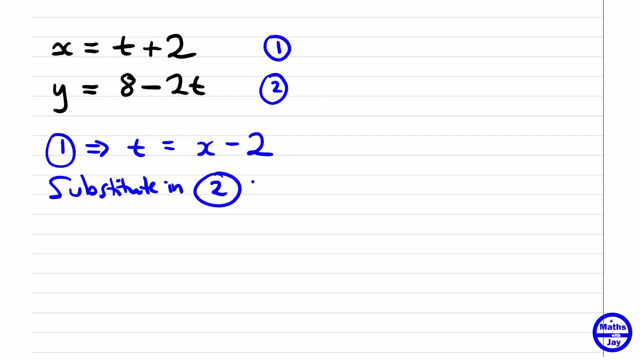 we'll bear that in mind. So let's start by numbering the equations 1 and 2, and what we're going to do is use the first one to make t the subject, and then we're going to substitute that into the second equation, so that where we see the t in the second equation, we're going to replace that by x minus 2.. 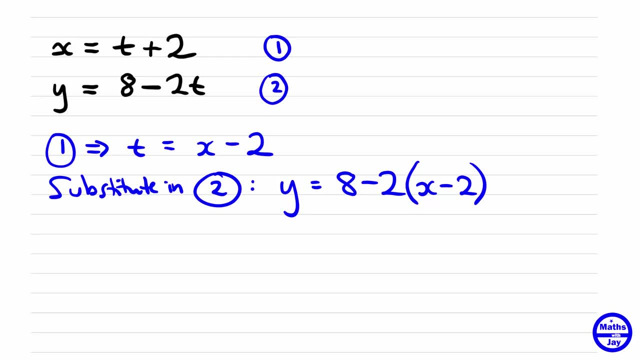 So you can see we have already eliminated t. So all we're going to do now is simplify this, so we're going to multiply out the brackets and add together the 8 and the 4.. So now we've got a nice equation. So there's our Cartesian equation, giving us y in terms of x, and we have eliminated t. 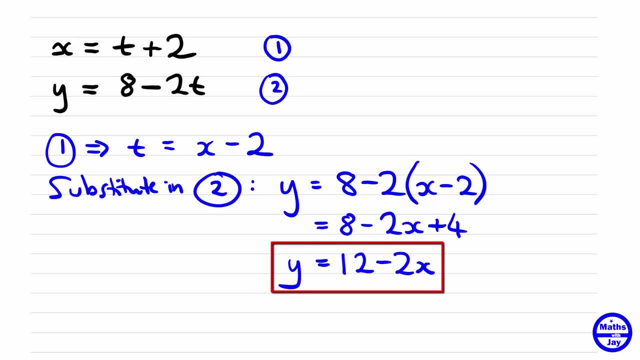 And you might like to check your answer. so what you could do is choose, maybe, um. what should we choose for t? to start with, let's choose the easiest value for t. So if we have a look at what happens when t is 0, if we use equation 1, we find that x is equal to 0. 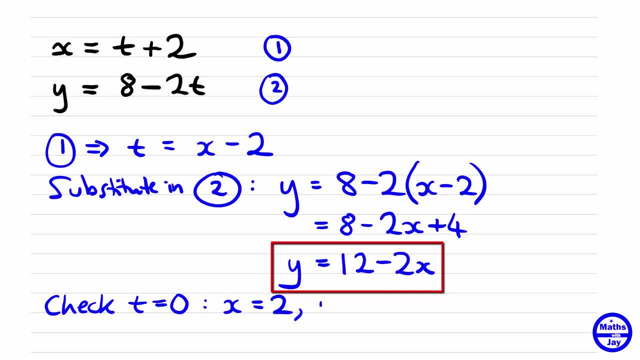 plus 2, so that's 2. and in equation 2, y is 8 minus 0, so y is 8, and what we're going to do is just check that y really is 12.. So we're going to subtract 2 times x, so let's have a look: 12 minus 2 times 2, so we're hoping that. 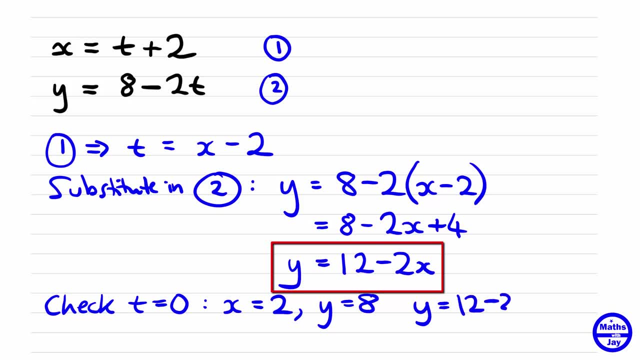 that will give us 8, which of course it does, doesn't it? so that is equal to 8. so that looks as if that's working. and we could check another value of t, um. what should we try? um 4. so if t is 4, 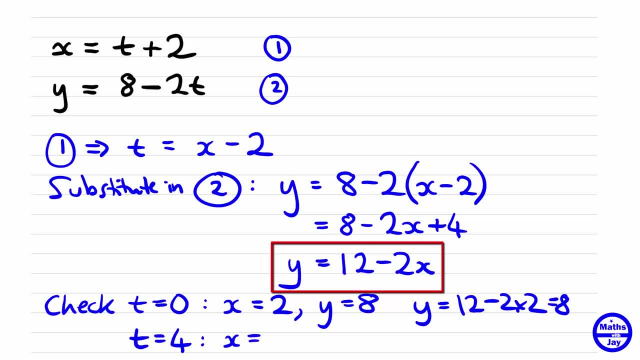 that would give us that x is 2.. Added on to 4, so that's 6, y would be 8 minus 2 times 4, so y would be 0. and using our Cartesian equation to check that it's giving the right answer, we've got 12 minus 2 times 6, so that is. 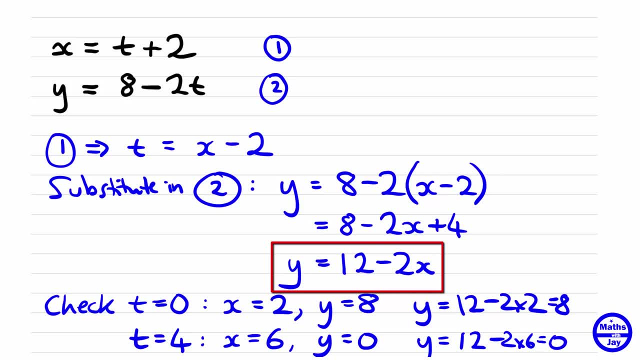 equal to 0, and so that shows that again our equation is working. so it looks like y is 12 minus 2x is correct.